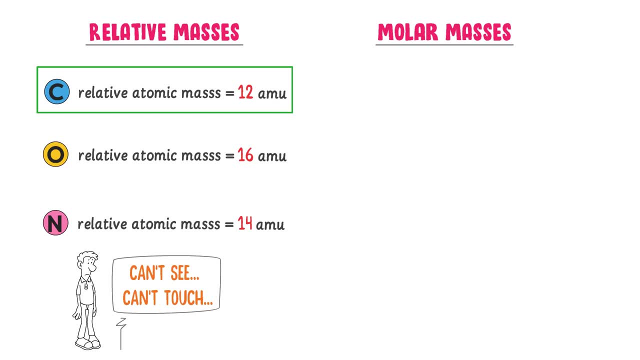 of a carbon atom. Now, to solve this issue, scientists put forward the concept of mole. For example, I cannot touch and see one atom of carbon or 12 amu of a carbon atom. Now, instead of 12 amu, I take 12 gm of carbon atom. We can see that in 12 amu of carbon there is 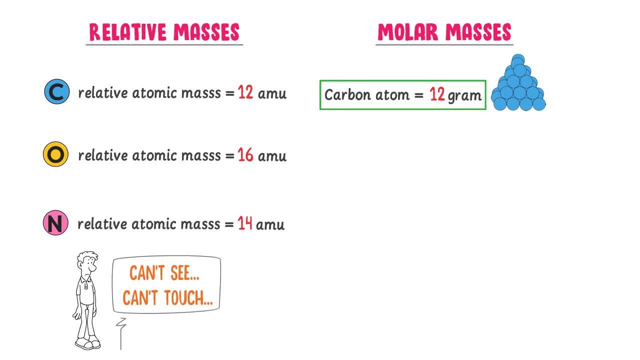 only one atom of carbon, While in 12 gm of carbon there are 6.023 x 10 to the power, 23 atoms of carbon are present. Similarly, instead of 16 amu of oxygen, we take 16 gm of oxygen and there are. 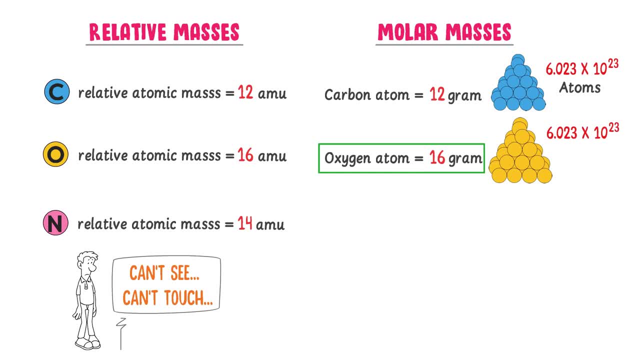 6.023 x 10 to the power, 23 atoms of oxygen are present in 16 gm. Also, instead of 14 amu of nitrogen, we take 14 gm of nitrogen and there are 6.023 x 10 to the power, 23 atoms of nitrogen. 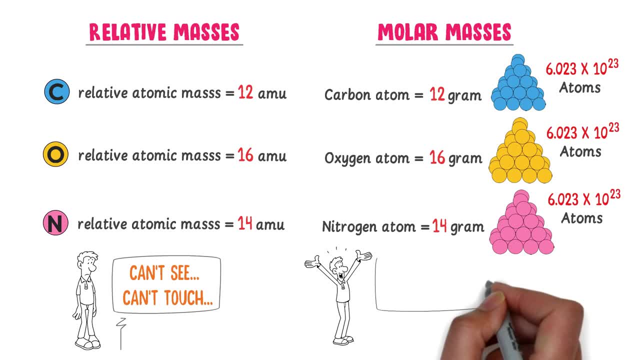 are present in 14 gm of nitrogen. Remember that now we can see, touch and do chemistry with 12 gm of carbon. Thus 12 amu, 16 amu and 14 amu are relative atomic masses, while 12 gm, 16 gm and 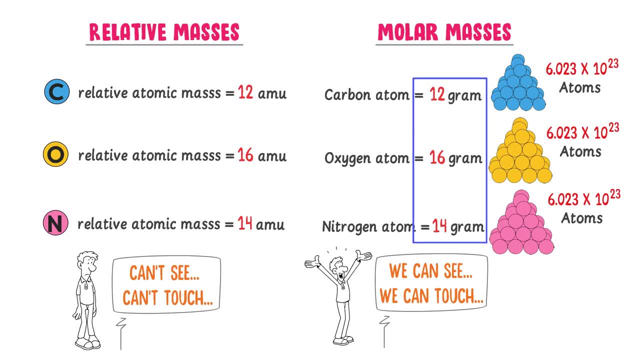 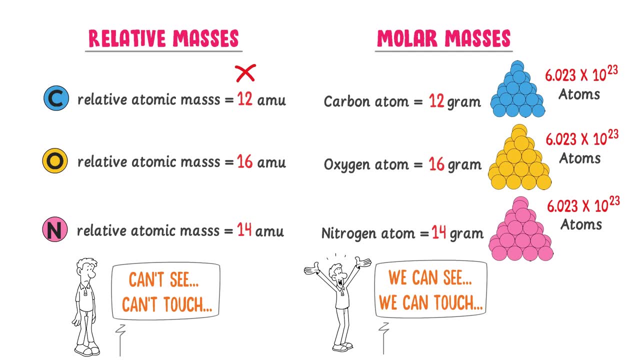 14 gm are molar masses or gram atomic masses. Therefore, note it down that to study mole concept we do not consider relative masses. We always play with molar masses. Here let me clear the biggest confusion of students: How 12 gm of carbon is relative to 12 gm of oxygen. 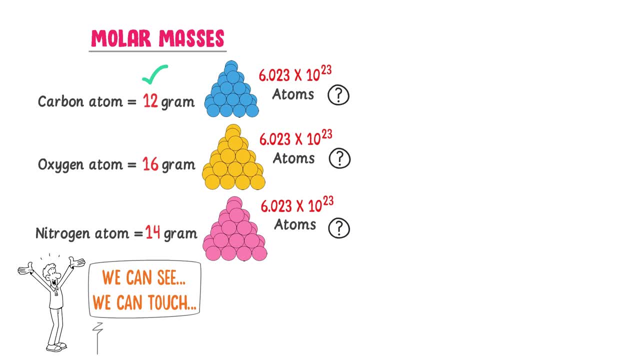 If 12 gm of carbon or 16 gm of oxygen or 14 gm of nitrogen is equal to 6.023 x 10 to the power 23 atoms, Well, if I ask you to give me one dozen pencils, how many pencils will you give me? 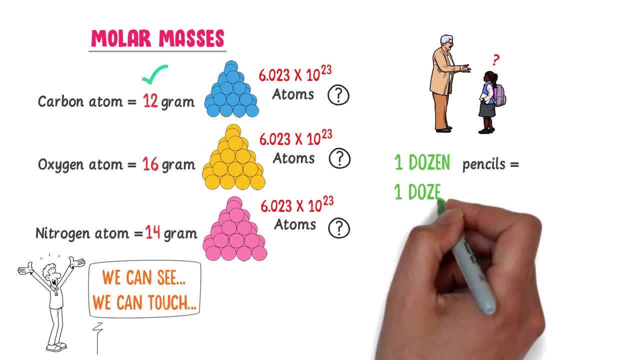 If I again ask you to give me one dozen eggs, how many eggs will you give me? Well, you will definitely say 12 pencils and 12 eggs, Because you know that one dozen pencils is equal to 12 pencils and one dozen eggs is. 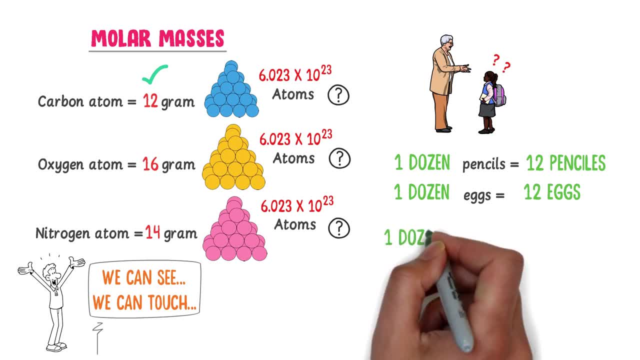 equal to 12 eggs. So we can write that one dozen of anything is equal to 12 items. Similarly, molar mass of any atom is equal to 6.023 x 10 to the power 23 atoms, Just like 12, 6.023. 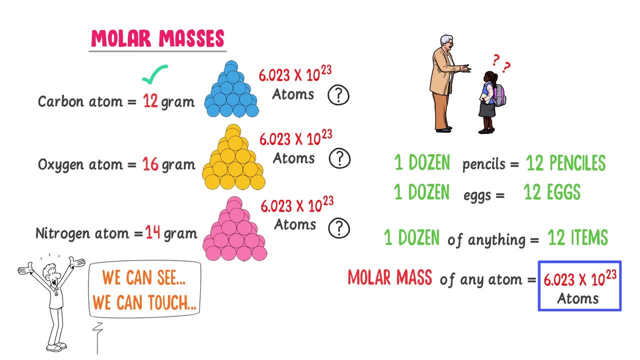 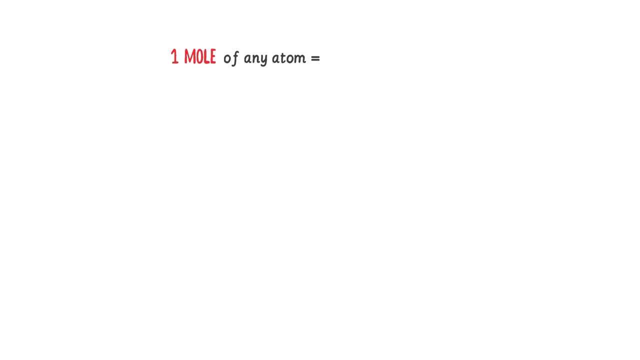 x 10 to the power, 23 is a simple number, Which is correct. It is commonly known as an Avogadro's number. Now listen carefully. One mole of any atom is equal to its molar mass. Let me repeat this important statement: One mole of any atom is equal to its molar mass. For example, 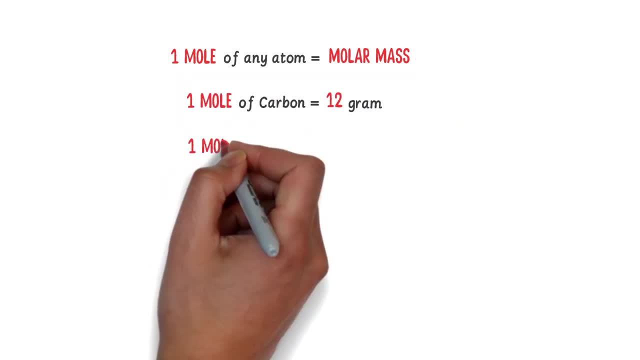 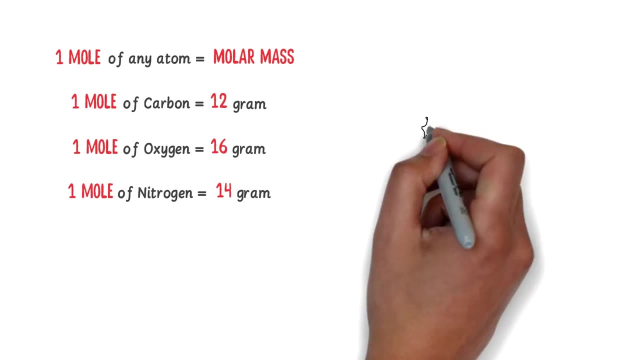 one mole of carbon atom is equal to 12 gm, one mole of oxygen atom is equal to 16 gm and one mole of nitrogen is equal to 14 gm. So if I ask you, Please tell me one mole of carbon, How many gm of carbon will you give me? 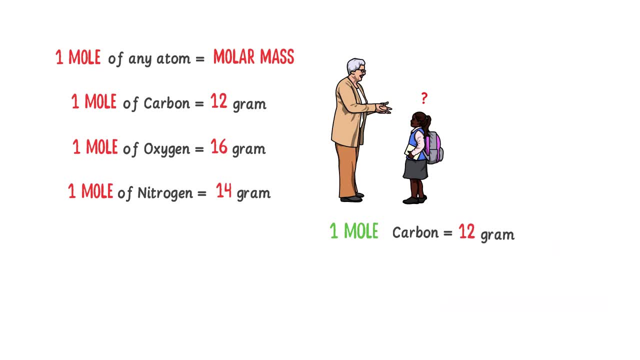 I hope you know the answer. You will definitely give me 12 gm of carbon, Because the molar mass of carbon is 12 gm. If I again ask you that how many atoms of carbon are there in one mole of carbon? Your answer is simple. 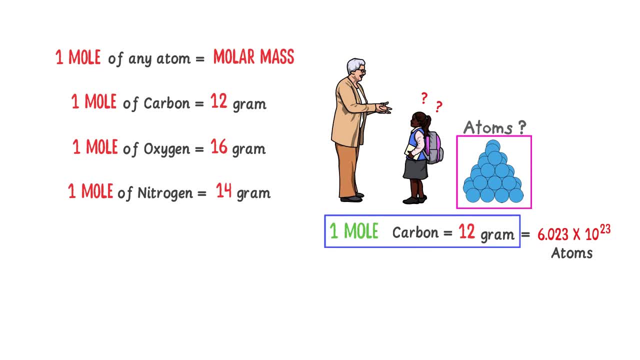 There are 6.023 x 10 to the power, 23 atoms of carbon are there and this one mole are there are 12 grams of carbon. Thus, in one mole of carbon there are 12 grams of carbon atoms, or there are 6.023 x 10 to the power, 23 number of atoms are present. It means we have to. 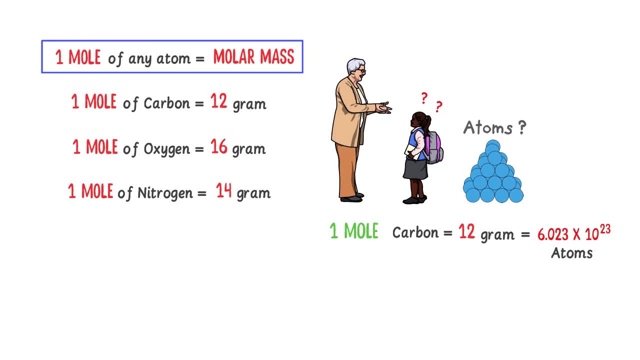 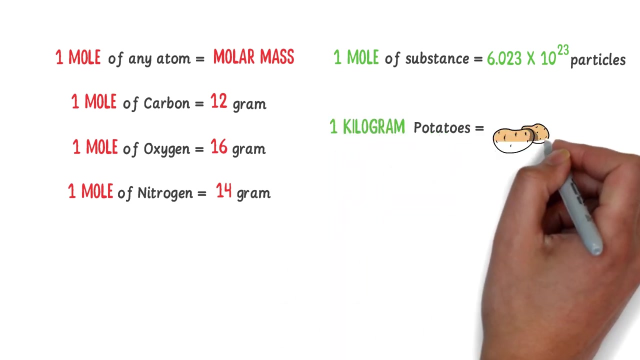 modify this definition of a mole. One mole is equal to molar mass, or one mole of any substance contains 6.023 x 10 to the power 23 particles. Here particles mean atoms, molecules or ions. If you are still confused, let me further explain it. Consider 1 kg potatoes. 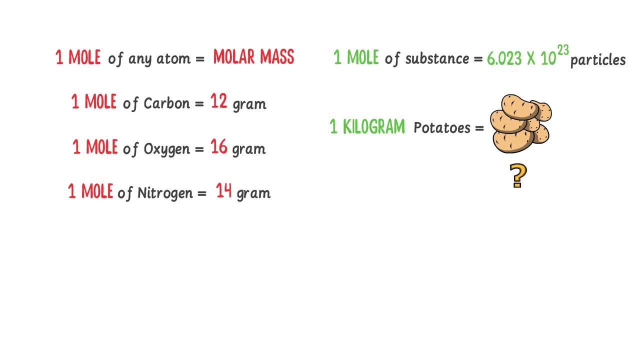 If I ask you how many potatoes are there in 1 kg, Well, you can count it and your answer is 6 potatoes. 1 kg is the mass of potato And in 1 kg there are 6 potatoes are present, And we can see that 6 is the simple number. 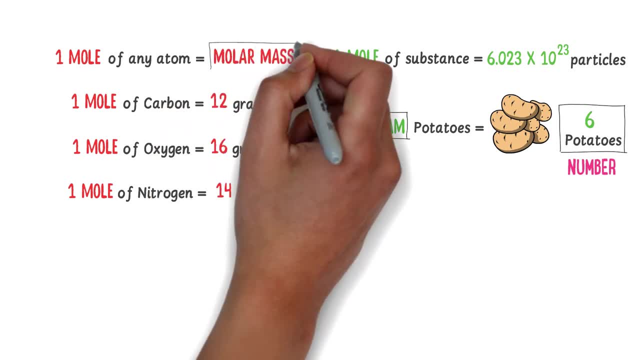 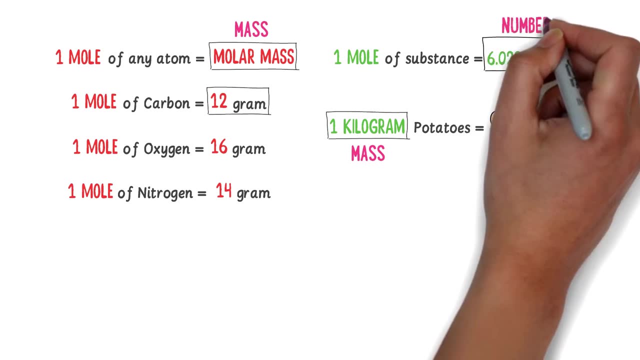 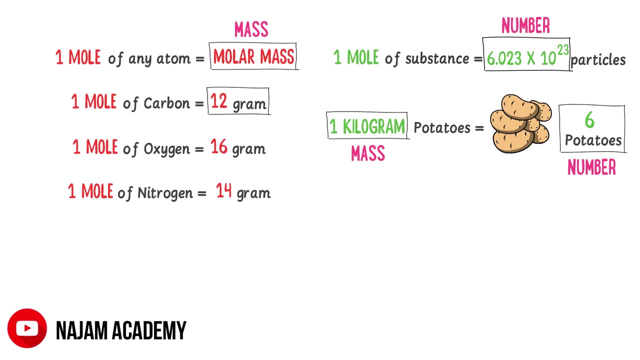 of potatoes. Similarly, 1 mole is the molar mass of any atom, like 12 grams of carbon. And in 1 mole there are 6.023 x 10 to the power, 23 atoms are present, So 6.023 x 10. 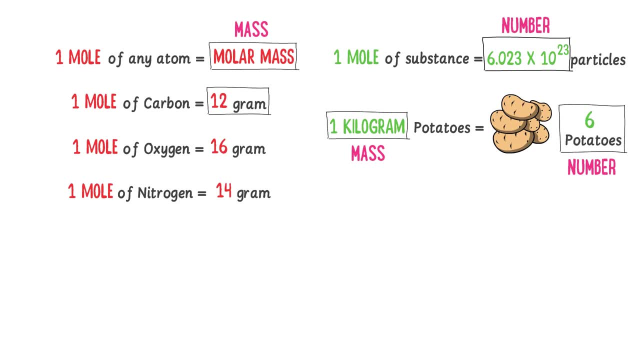 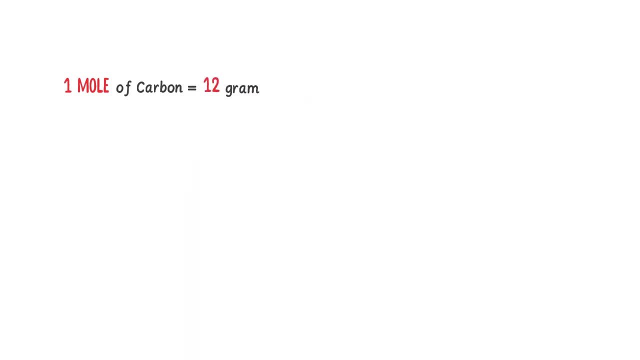 to the power, 23 is a number, just like a 6.. To summarize, as the mole concept, we can say that 1 mole of carbon atom is equal to 12 grams. Secondly, in 1 mole of carbon there are 6.023 x 10 to the power, 23 atoms of carbon are present. 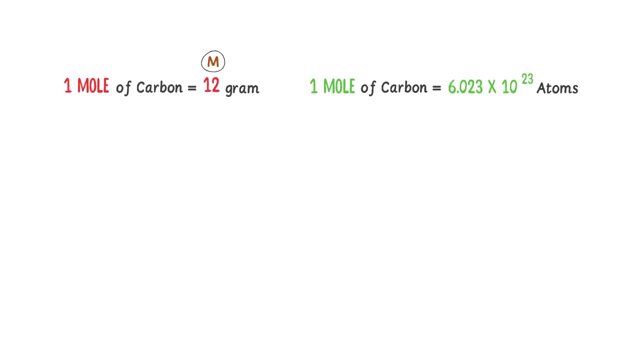 So we say that this is mass-M relationship and this is number-N relationship. Secondly, 1 mole of oxygen atom is equal to 16 grams. This is M relationship. 1 mole of oxygen atom contains 6.023 x 10 to the power, 23 atoms of oxygen. This is N relationship. 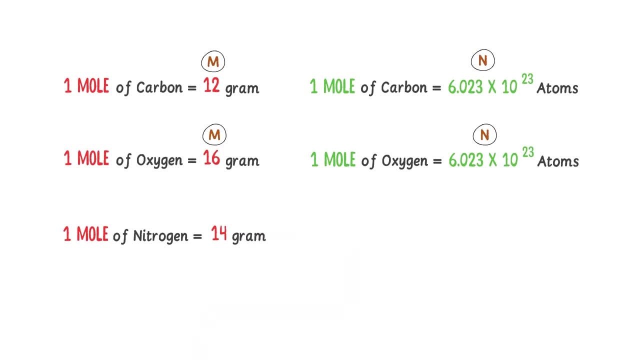 Thirdly, 1 mole of nitrogen atom is equal to 14 grams. This is M relationship. In 1 mole of nitrogen atom there are, 6.023 x 10 to the power, 23 atoms of nitrogen. This is N relationship. Now I will use M relationship and N relationship to calculate the mass of. 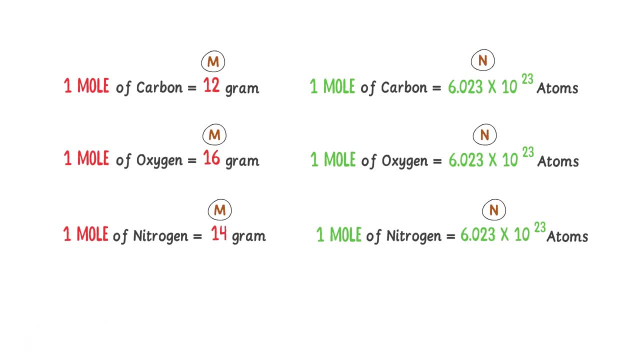 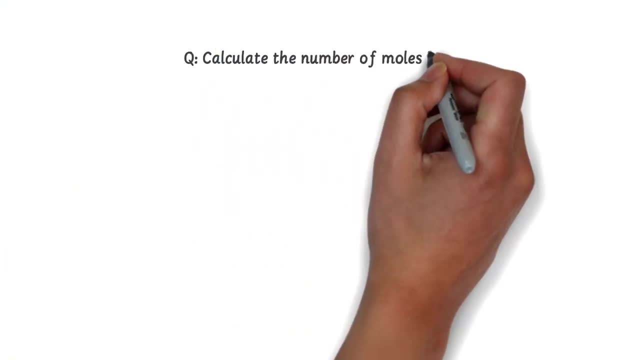 M-Mole fluid in the atom. These are the N-moles of M-Mole fluid. If you have any questions, please ask us in the comment section. Now. also note down the number of moles in the atom. For example, calculate the number of moles in 32 grams of oxygen atom. 16 grams of carbon. 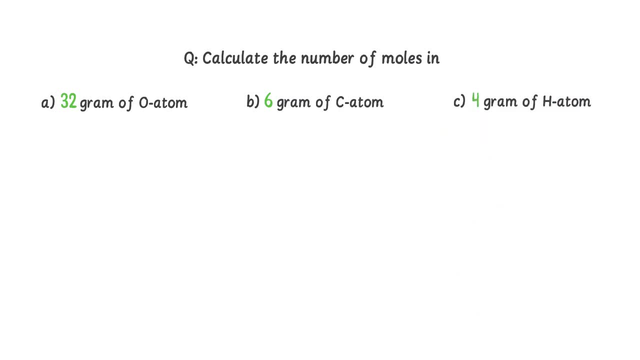 atom and 4 grams of hydrogen atom And the question: we are given masses of the different atoms. so in this type of numericals always write M: relationship of moles. We know that 1 mole of oxygen atom contains 5.023 x 10. to the power 23,. and this number of moles is 7.024 x 10 to the power 9.5.. So we know that 1 mole of oxygen atom contains 6.023 x 10 to the power 26 atoms of hydrogen. This is N relationship. 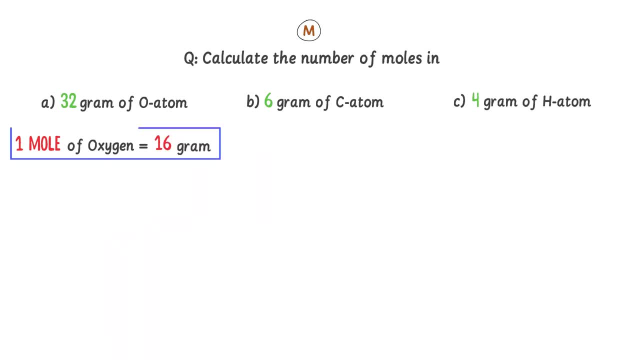 is equal to 16 grams. Just like this relationship. we can say that let x moles are there and 32 grams Now cross. multiply them, I get 16 into x is equal to 32 into 1.. Dividing both sides by 16, I get x is equal to 2 moles. So there are 2 moles of oxygen atom are present. 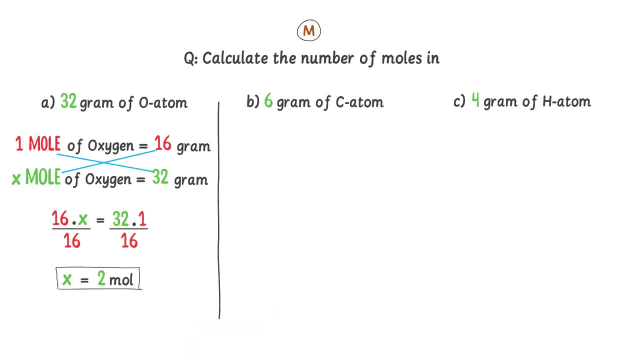 and 32 grams. Secondly, in case of carbon, 1 mole of carbon atom is equal to 12 grams. Let x moles are there and 6 grams of carbon Now cross. multiply them, I get 12 into x is equal to 6 into 1. Dividing both sides by 12, I get x is equal to 0.5 moles. So there, 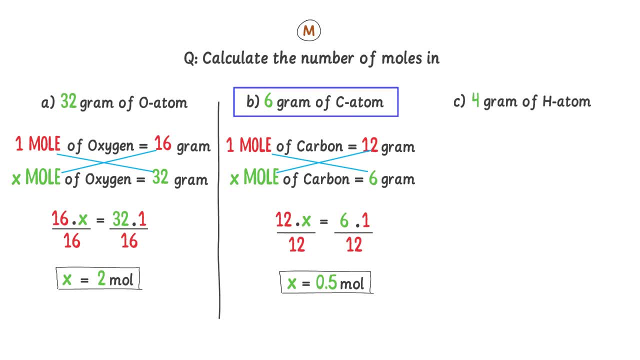 are 0.5 moles are present and 6 grams of carbon. Thirdly, in case of hydrogen, I get: 1 mole of hydrogen is equal to 1 gram Let x moles are there and 4 grams of hydrogen. 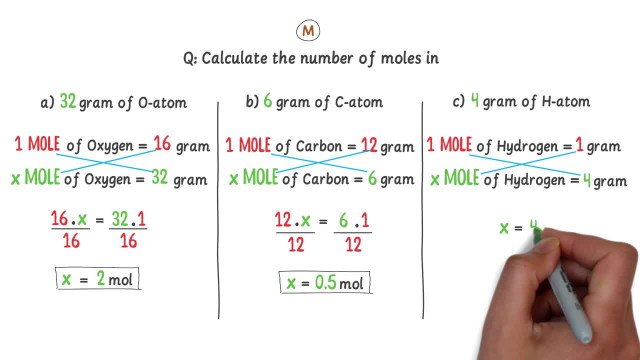 Now cross, multiply them, I get: x is equal to 4.. So there are 4 moles of hydrogen are present and 4 grams. Therefore, in such type of numericals we use m-relationship to calculate the number of moles. Also, let me teach you the second type of calculation: Calculate. 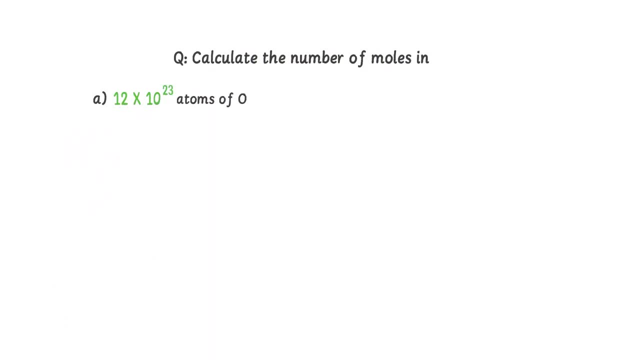 the number of moles and 12 into 10 to the power 23.. So I use 6 into 10 to the power 23 atoms of oxygen and 18 into 10 to the power 23 atoms of carbon. Rest 2 radians are given and they are given. 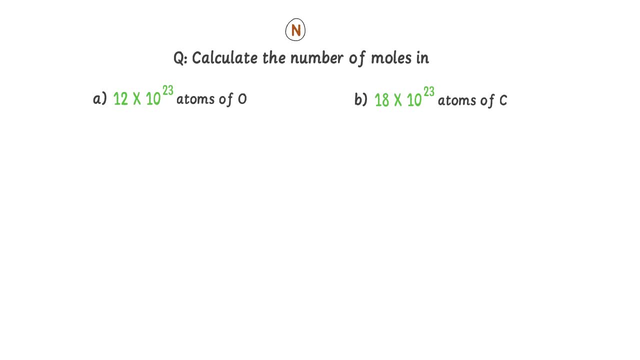 m-relationship to create the 10- laziness contract. Now, in case of oxygen, we say that 1 mole of Oxygen atom contains 6 into 10 to the power 23 atoms. Note down that I use 6 into 10 to. 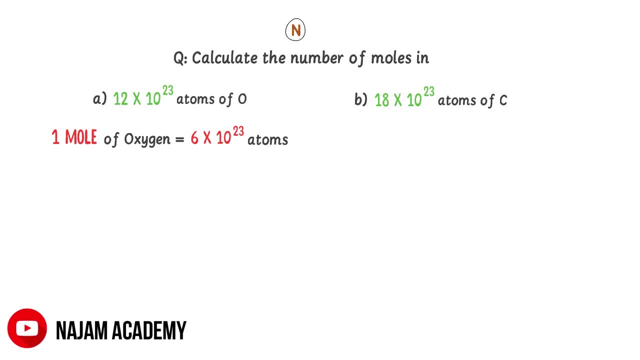 the power 23,. not 6 Moles. Not implementation means meltliization. mass volume: 0 to 3 into 10 to the power 23. just for easy calculation, Let an x mole- there are 12 into 10 to the power 23. atoms of carbon are present. 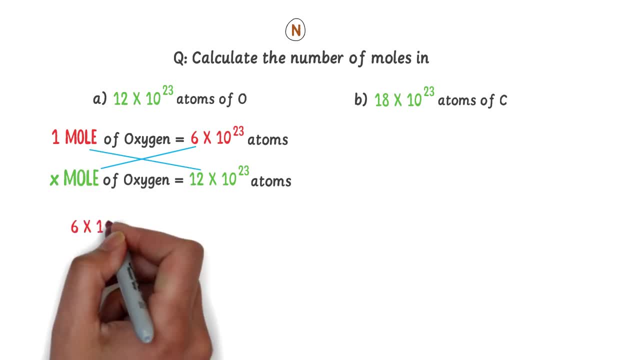 Now cross. multiply them, I get 6 into 10 to the power 23 into x is equal to 12 into 10 to the power 23 into 1. Dividing both sides by 6 into 10 to the power 23,, I get 2 moles. 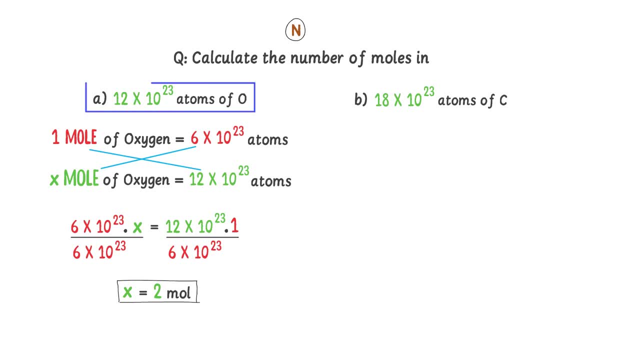 So there are 2 moles of oxygen are present and 12 into 10 to the power 23 atoms. Secondly, in case of carbon, one mole of carbon contains 6 into 10 to the power 23 atoms. Let an x mole, there are 18 into 10 to the power 23 atoms of carbon are present. 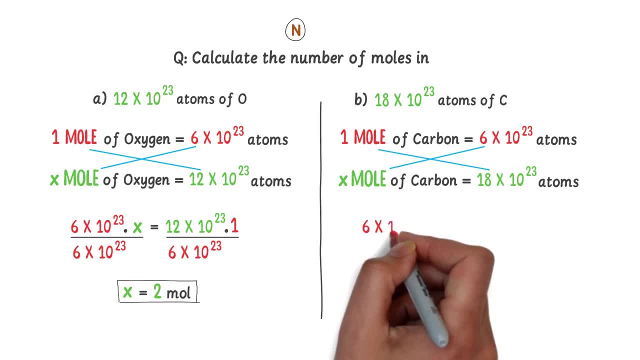 Now cross. multiply them, I get 6 into 10 to the power 23 into x is equal to 18 into 10 to the power 23 into 1. Dividing both sides by 6 into 10 to the power 23,, I get 3 moles. 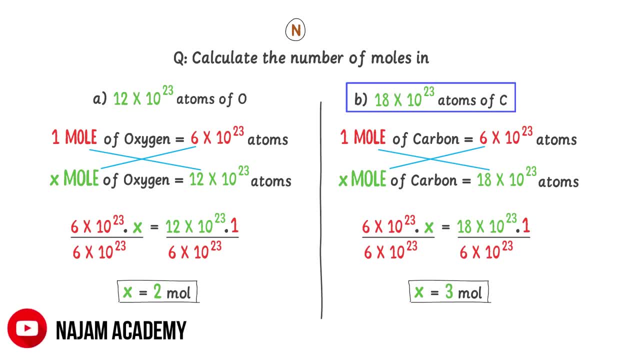 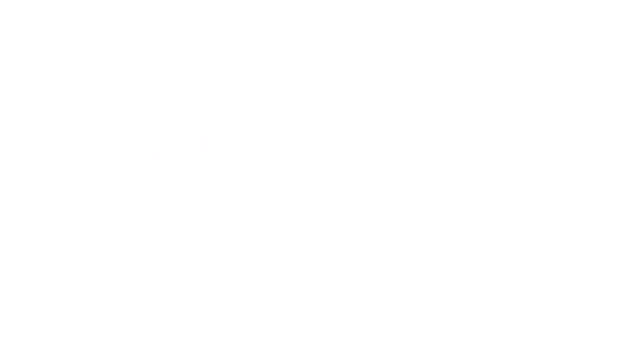 So there are 3 moles of carbon are present and 18 into 10 to the power, 23 atoms of carbon. Therefore, in such type of numericals, always use the number and mole relationship to calculate the number of moles. Now let me take you to the medium level. 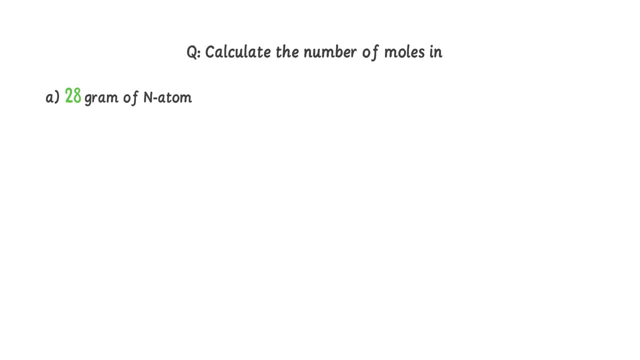 Calculate the number of moles in 28 gm of nitrogen atoms. Let me take you to the medium level. I get a small intact辑- at least student- from Made in America. Divid 1. 0 speaks for 8 moles and 8 y regular 0 speaks for 9 moles. 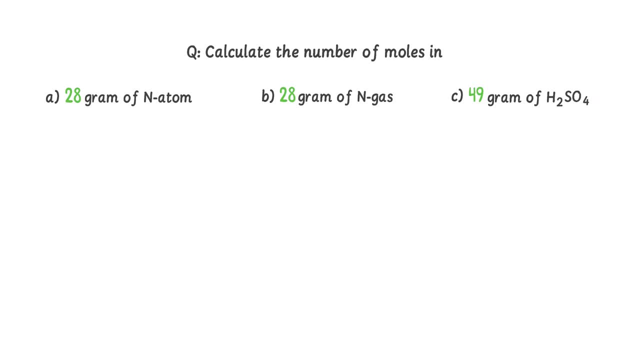 Divid 1 by 11 by 11 is equal to 18 y H2SO4.. Add an x to the power, 20 kN, then there are 28 gm of nitrogen gas and 49 gm of H2SO4. 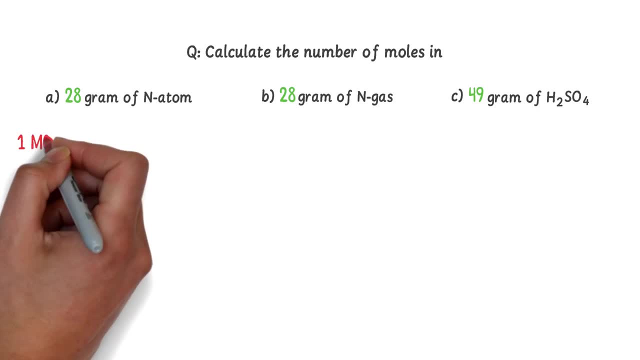 In case of nitrogen atom, we know that one mole of nitrogen atom is equal to 14 gram, So there are x moles present and 28 gm of nitrogen. After calculation, I getn is equal to 2 moles, So there are 2 moles present and 28 gm of nitrogen. 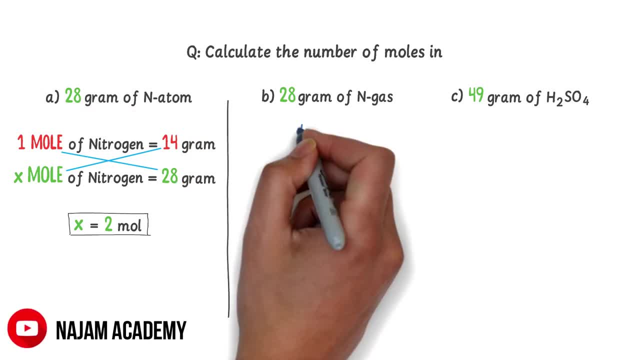 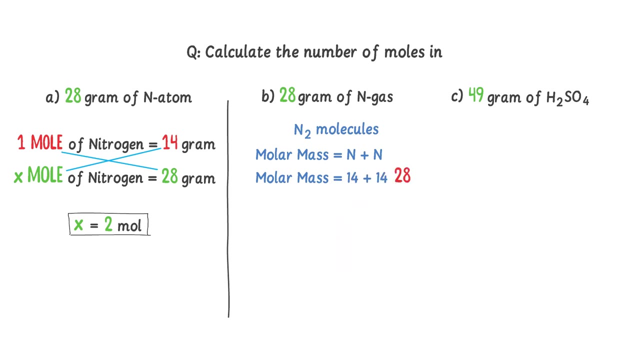 While n the case of nitrogen gas, we know that there are N2 molecules are present in the nitrogen gas. First of all I need to find the molar mass of N2 molecules. I write N plus N are 14 plus 14 and I get 28 gram. 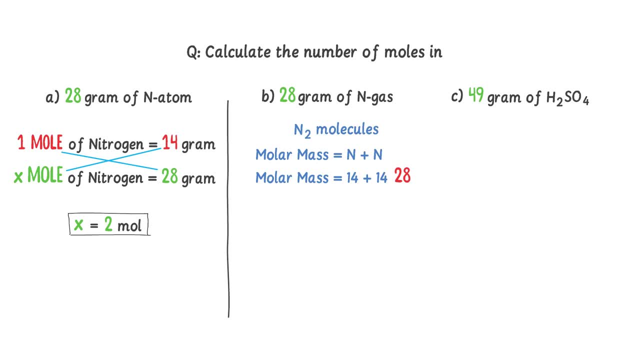 So the molar mass of N2 molecules is 28 grams. Hence we say that one mole of nitrogen gas is equal to 28 grams. Let there are X moles present in 28 grams of nitrogen gas. After calculation I get one mole. 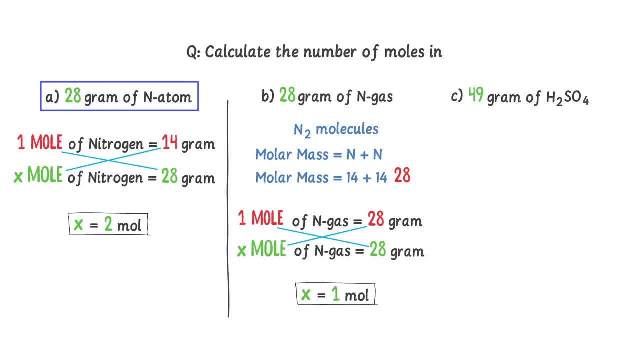 Thus remember that in 28 gram of nitrogen atom there are two moles present of nitrogen, While in 28 gram of nitrogen gas there is only one mole of nitrogen gas is present. Thirdly, in the case of 49 gram of H2SO4,, first of all I need to find the molar mass.